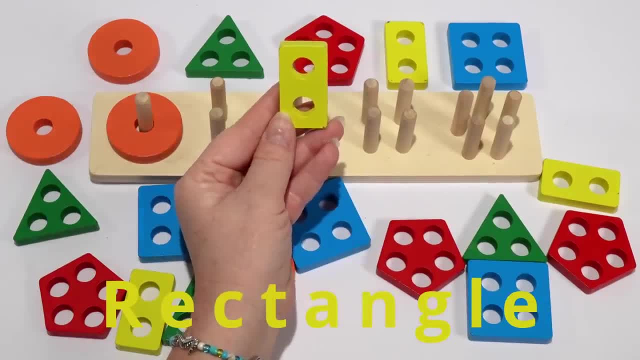 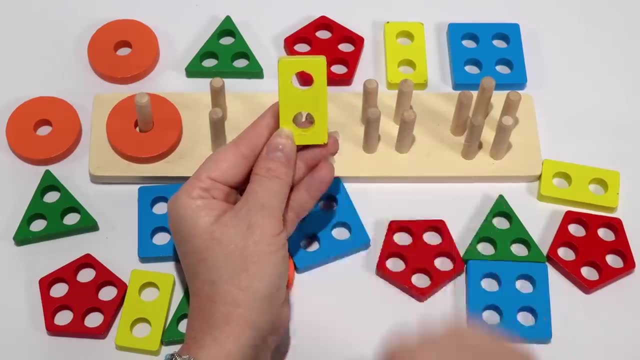 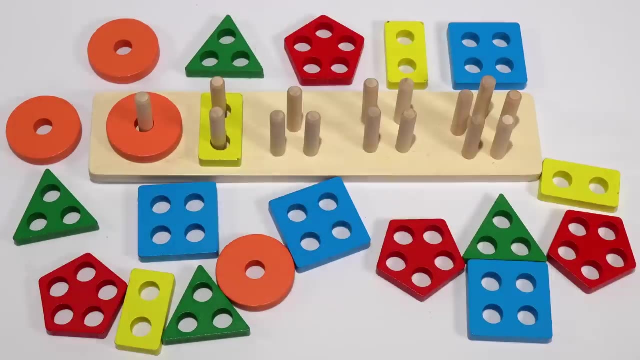 Does our rectangle have only two holes? That's right, our rectangle has two holes, One, two and our rectangle is yellow. Our next set has one, two, three pegs. We know what shape has. only three holes. we just looked at it. 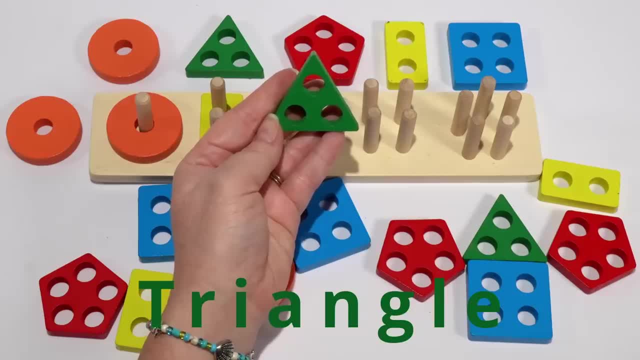 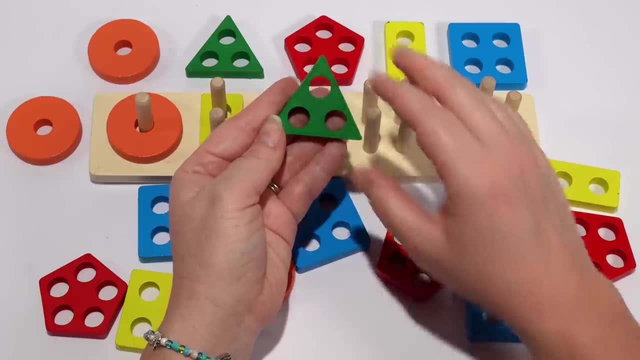 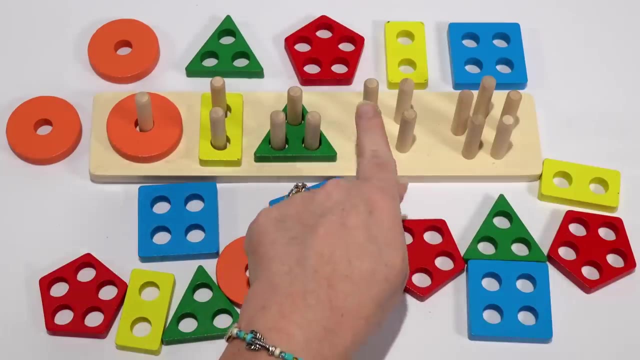 It's our triangle. Our triangle is green and it has one, two, three holes. Our next set of pegs has one, two, three, four. Do you see a shape that has four holes? Does this one have only four holes? 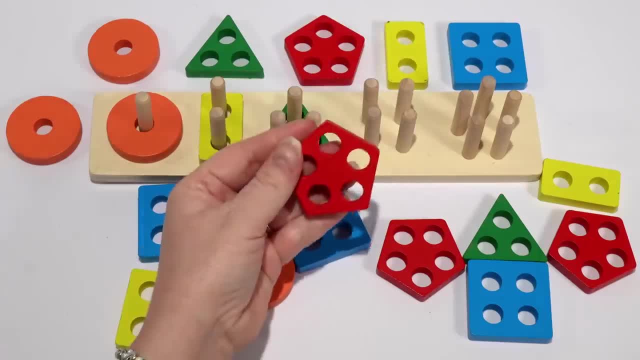 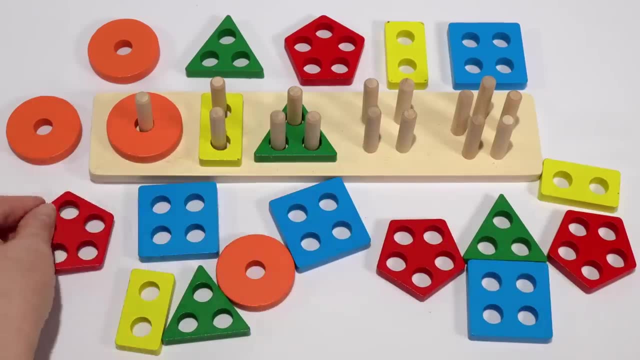 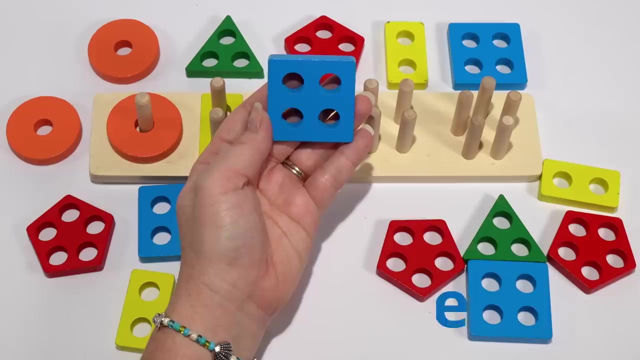 No, it has one, two, three, four, five. So it must be our square. Our square has four holes: One, two, three, four. And our square is blue. Our square has four holes: One, two, three, four. 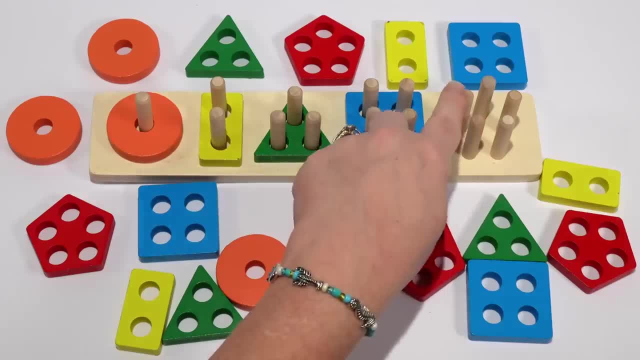 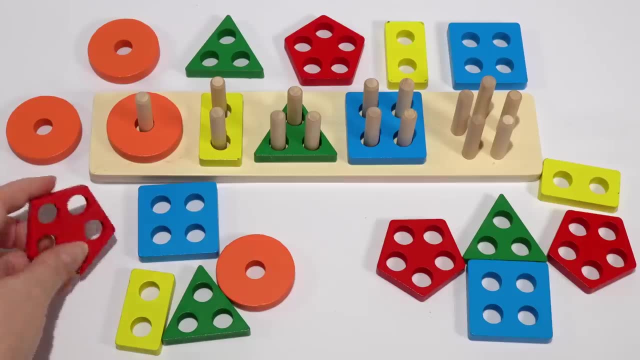 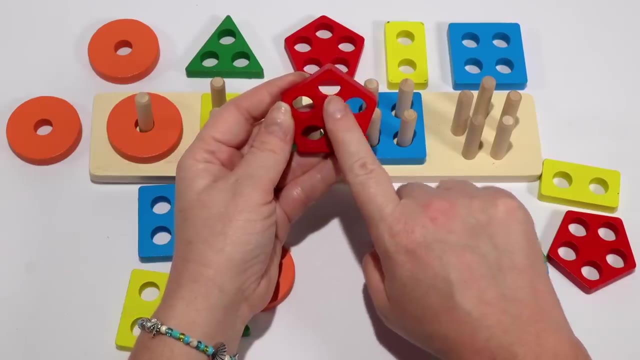 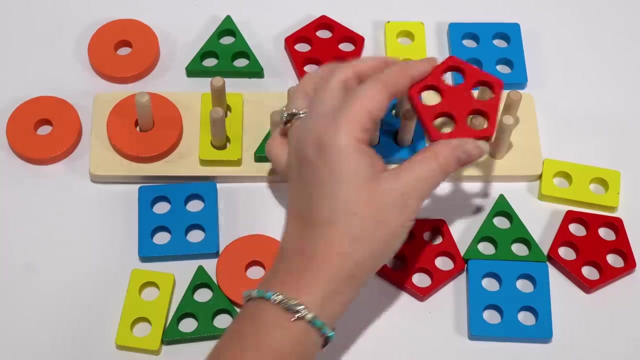 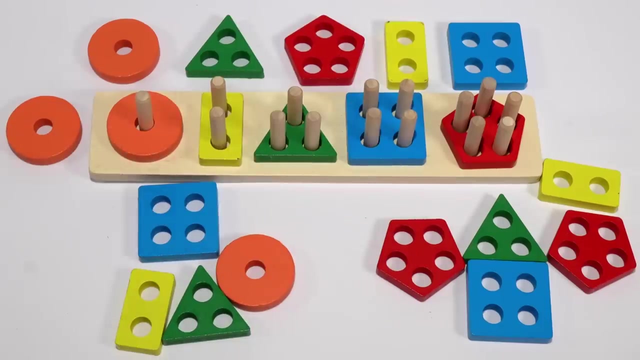 Our last set of pegs has one, two, three, four, five, And thisекс, our pentagon, has five holes: One, two, three, four, five. Our pentagon is red, So we have an orange circle. Let's count the rest of our orange circles. We have one, two.